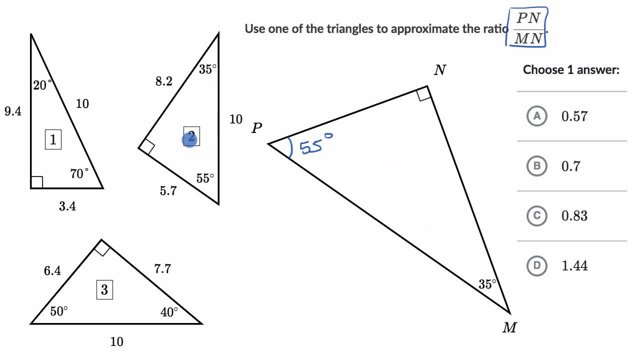 between triangle PNM and triangle number two right over here. we know that these two are similar triangles, And so the ratios between corresponding sides are going to be the same. We could either take the ratio across triangles or we could say the ratio within, when we just look at one triangle. 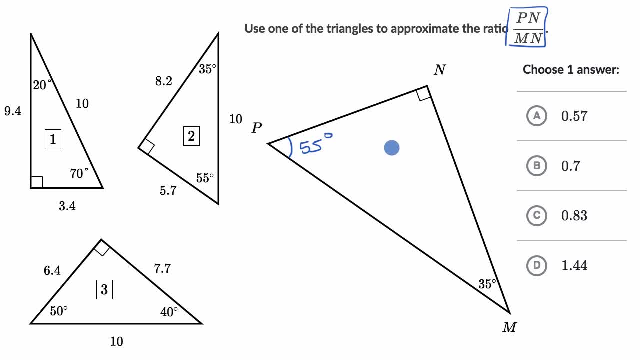 And so if you look at PN over MN, let me try to color code it- So: PN right over here, that corresponds to the side that's opposite, the 35 degree angle. So that would correspond to this side, this side right over here on triangle two. 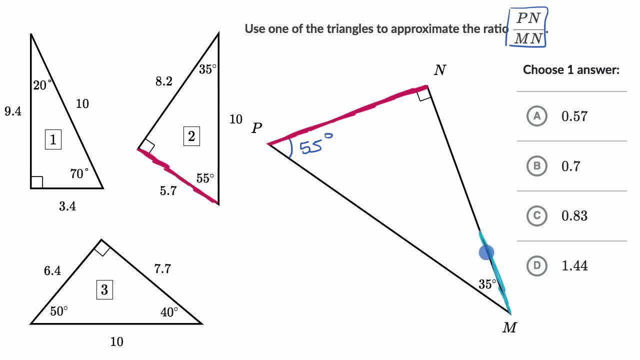 And then MN, that's this that I'm coloring in this bluish color. not so well, probably spend more time coloring That's open, that's opposite the 55 degree angle, And so opposite the 55 degree angle would be right over there. 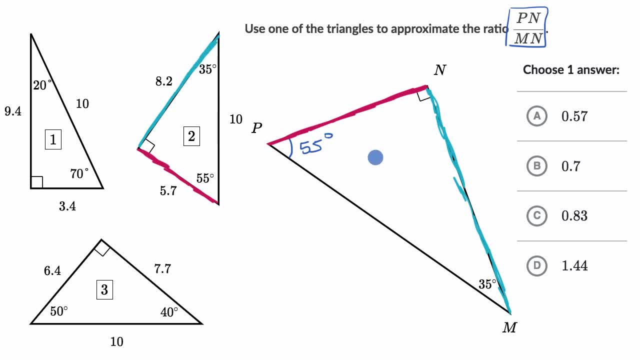 Now, since these triangles are similar, the ratio of the red side, the length of the red side- over the length of the blue side, is going to be the same in either triangle. So PN- let me write it this way- The length of segment PN over the length of segment MN. 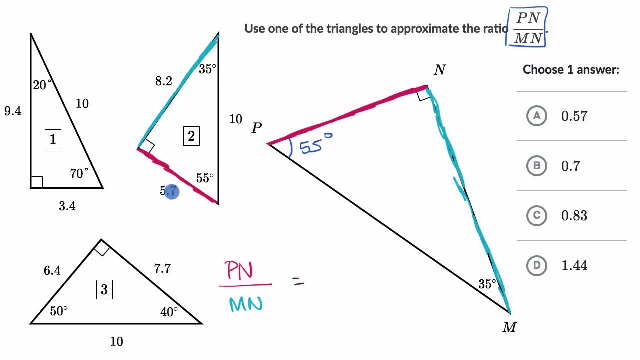 is going to be equivalent to 5.7 over 8.2, because this ratio is going to be the same for the corresponding sides, regardless of which triangle you look at. So if you take the side that's opposite, 35 degrees. 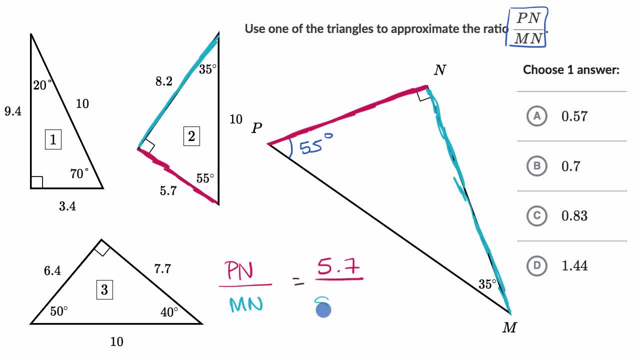 that's 5.7 over 8.2.. Now, to be very clear, it doesn't mean that somehow the length of this side is 5.7 or that the length of this side is 8.2.. We would only be able to make that conclusion. 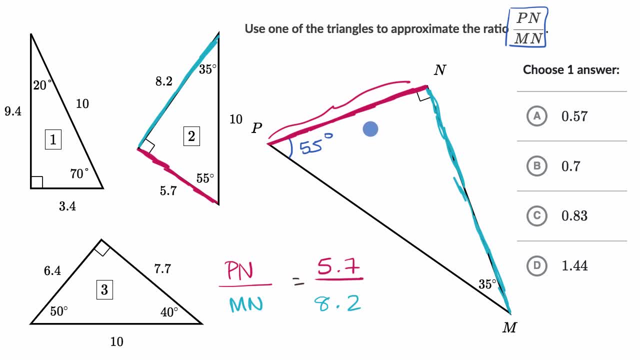 if they were congruent, But with similarity. we know that the ratios, if we look at the ratio of the red side to the blue side on each of those triangles, that would be the same, And so this gives us that ratio, And let's see 5.7 over 8.2,. 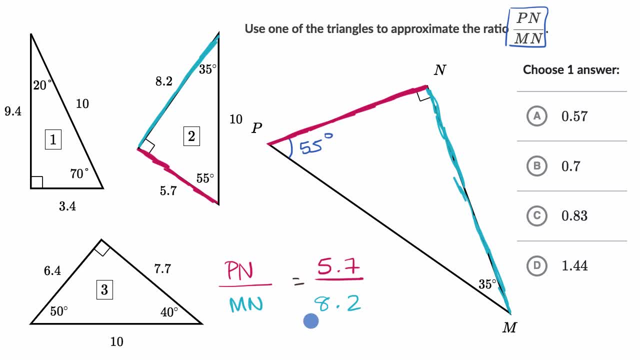 which of these choices get close to that? Well, we could say that this is roughly well. we could say that this is roughly well. we could say that this is roughly. if I am approximating it, let's see, it's going to be larger than 0.57.